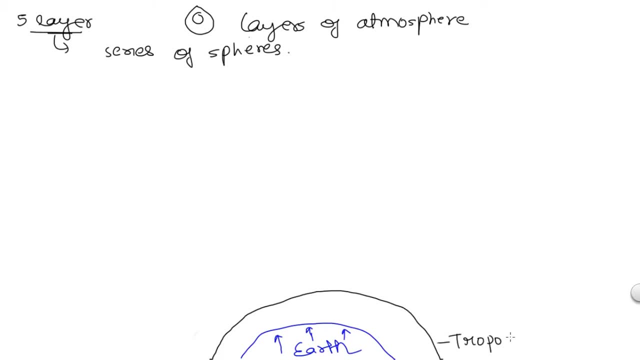 surface is called troposphere. Second layer is called stratosphere, which is lying above the troposphere. Third layer, which is lying above the stratosphere, is called mesosphere. Fourth layer is called thermosphere, and the fifth and last layer is called exosphere. So these are the five. 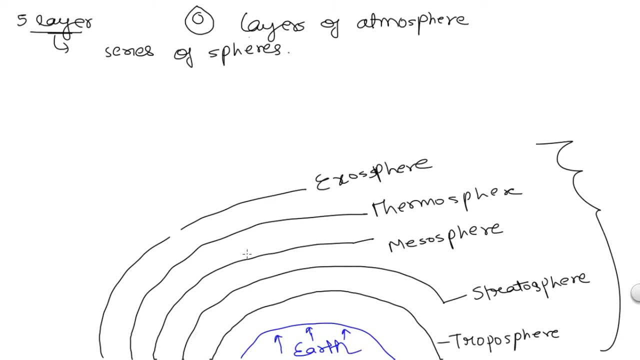 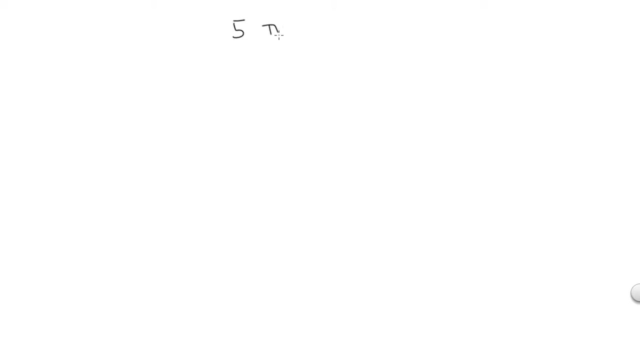 layers which are forming your atmosphere, which is looming around the earth surface because of its gravitational pull. These five layers are also called as thermal layers. Thermal is signifying the temperature gradient or temperature profile, which means these layers have been divided based on their temperature gradient. These five thermal layers can be grouped as homosphere. 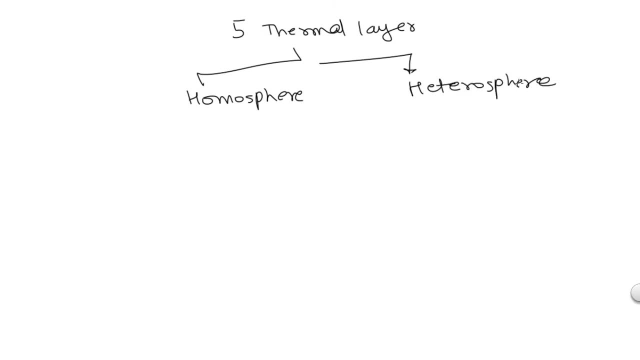 and heterosphere. Here homo means homogeneous, which means there is uniform mixing of gases. uniform mixing of gases in homosphere, whereas in heterosphere there is non-uniform mixing of gases. The three lower layers, that is, troposphere, stratosphere and mesosphere. These three layers: 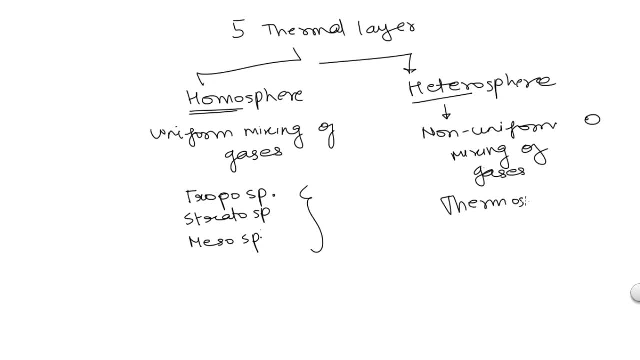 come under homosphere, whereas thermosphere comes under heterosphere, where there is non-uniform mixing of gases. So this was about thermal layers. Each layer has different name, different role, different composition, and each layer is located at different height above the earth surface. Let's talk about these layers one by one. So first we are going to talk about troposphere. 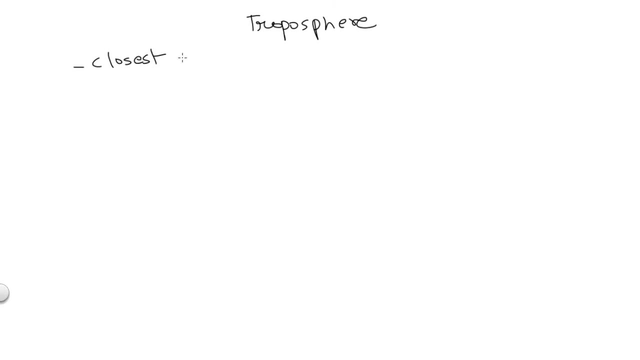 troposphere is the lowest layer, or the layer closest to the earth. Troposphere is the lower layer, or the layer closest to earth surface. So the first layer is troposphere. Troposphere can be discussed based on three points. So first is depth or thickness of troposphere. Second is temperature. 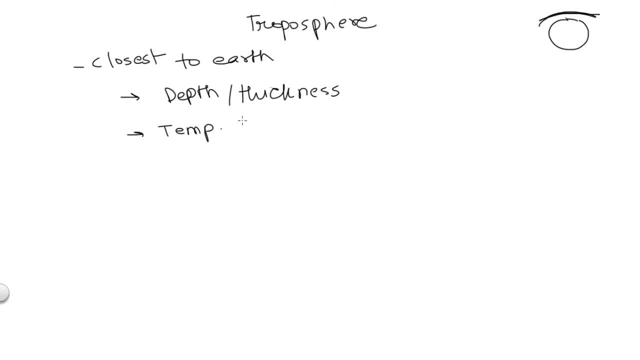 gradient of troposphere. that means how temperature is behaving when you go up above the earth surface. and third point is composition of troposphere. We will start with depth or thickness of troposphere. On an average, the troposphere lies up to 10 kilometers above the earth surface. So suppose this is your earth. when you go up above the earth surface till 10 kilometers you will find your troposphere. This height of troposphere varies when you move from equator towards the pole. So at equator the thickness of troposphere is different from the thickness of troposphere. At equator troposphere is much thicker than the troposphere at poles, So you can say the thickness is deeper at equator, where thickness of troposphere is shallower at poles. Let's talk about the reasons why there is difference in the thickness of troposphere when you move. 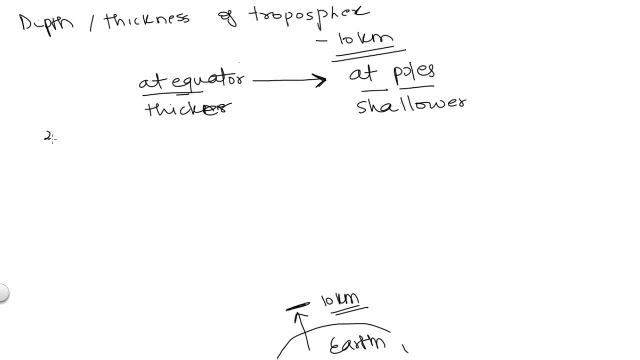 from equator towards the pole. So there are basically two reasons: First is temperature difference and second is temperature. So let's talk about the difference in temperature difference. So let's talk about the difference in temperature difference. So first we are going to talk about the temperature, As all. 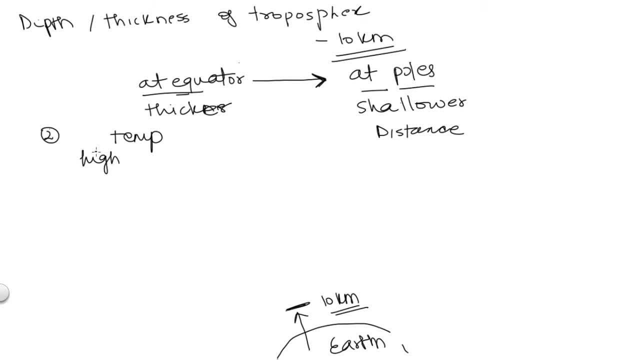 of you know, at equator we have higher temperature. Because temperature is high, that means air is warm above the equator and, as all of you know, warm air is less denser Because it is lighter. warm air rises up quickly in the atmosphere. Because of this warm air, the troposphere expansion. is happening above the equator. so troposphere is expanding and it extends up to 18 kilometers, whereas if you talk about the poles, you will find the temperature is lesser. that means air is cold, and cold air is denser and heavy air cannot rise up, rather it tries to sink. so this is your equator. 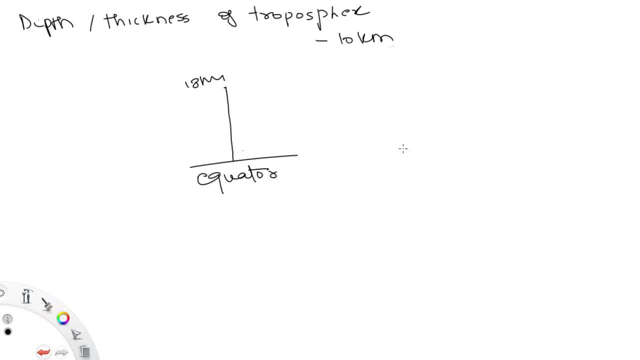 where the troposphere extends up to 18 kilometers, whereas at the poles, your troposphere is extending up to 8 kilometers. so what is happening at equator? the temperature is higher. because of high temperature, air gets heated up and warm air rises up in the atmosphere. because warm air is. 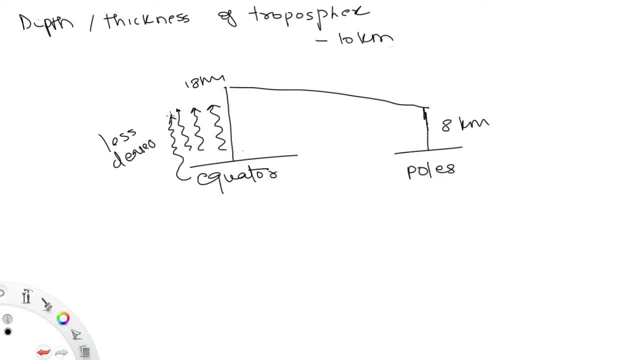 less denser. because of this upward movement of warm air, the troposphere expansion is happening above the equator. so troposphere is expanding above the equator, whereas if you talk about poles, what is happening here? the temperature is less. because of less temperature, cold air prevails. 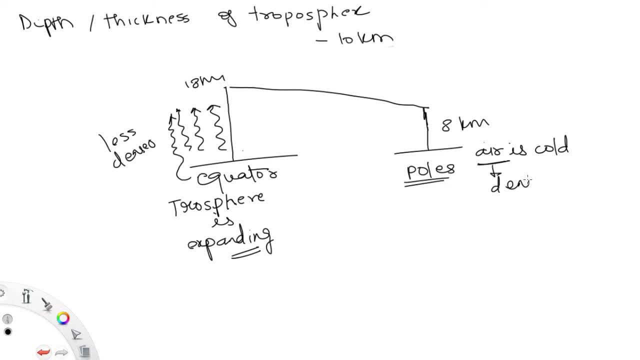 above the poles. cold air is denser in nature and because it is heavy it cannot rise, rather it tries to sink. so the cold air tries to sink, whereas warm air tries to rise up. because cold air is sinking down, that leads to troposphere contraction. so troposphere is contracting above the poles. this is one reason why the thickness of troposphere decreases when you move from equator towards the pole. other reason behind this thickness variation of troposphere can be distance of pole and equator from earth core, and this is because your earth is not spherical in shape. 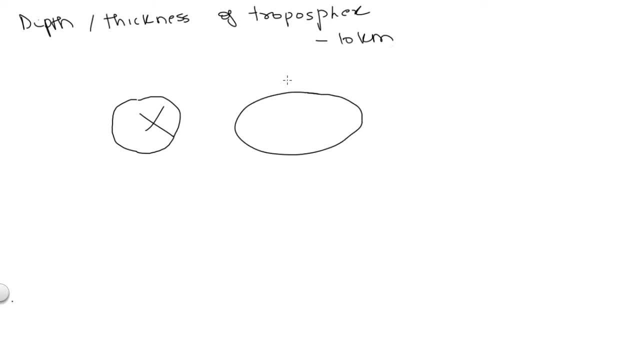 rather it is elliptical. so if this is your earth, poles are here and equator is lying here. you can see the polar radius is much lesser than the equatorial radius. that means the poles are closer to earth, closer to earth's core. because poles are closer to earth's core, poles are experiencing. 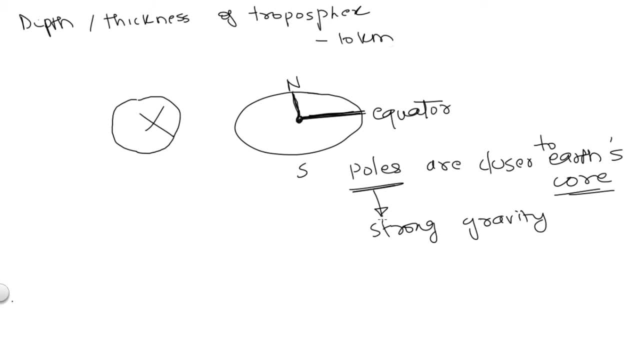 strong gravitational force, or you can say earth is exerting strong gravitational pulls at the poles and because of this higher gravitational force, the troposphere above the poles starts contracting, whereas if you talk about equator- because equatorial distance or equators are located farther away from the earth's core- 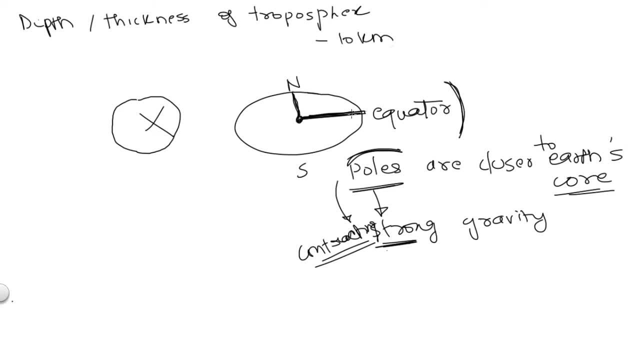 that is why the equatorial regions are experiencing weak gravitational force and because there is weak gravitational pull at the equator, the troposphere tries to expand. these are the two reasons why the thickness varies when you move from equator to poles. let's talk about the temperature gradient of troposphere, which means how temperature is behaving. 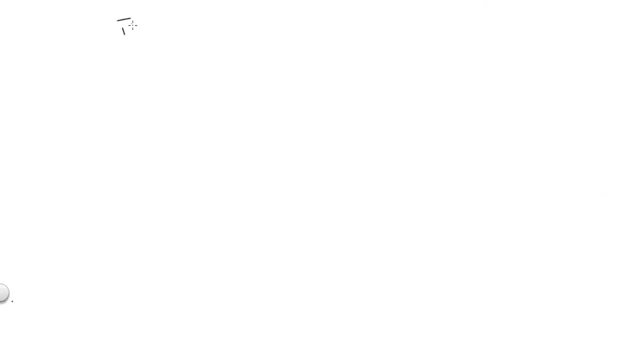 when you move up above the earth surface to understand the temperature gradient of troposphere. so in the temperature profile of troposphere let me draw a graph. so here x-axis is denoting temperature and y-axis is denoting your altitude in kilometers. so what is happening when you move up in this troposphere? your temperature starts. 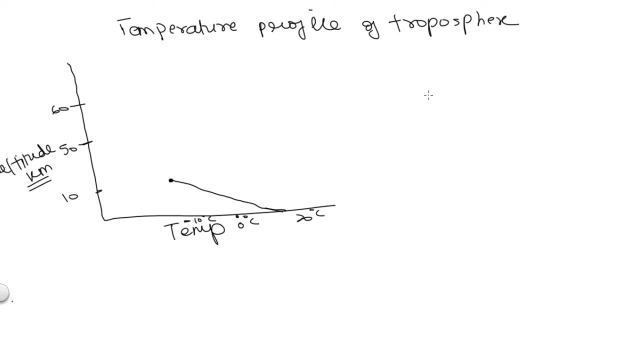 decreasing temperature starts decreasing- this decrease in temperature or this change in glider. so later here x-axis is referring to how temperature is changing in the troposphere. so in troposphere this change in temperature is called lapse rate. so lapse rate is of course denoting how temperature is changing when you move up in the atmosphere. so in troposphere temperature. 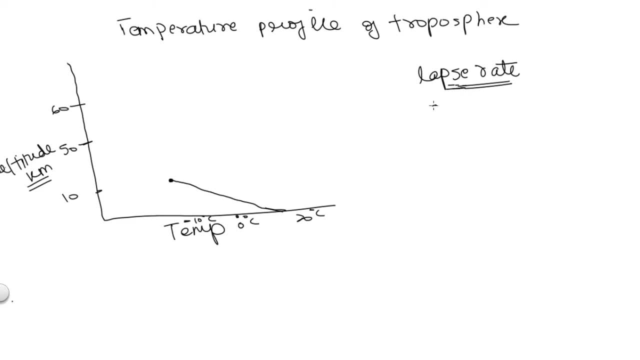 starts decreasing as you increase the height. this lapse rate can also be called as environmental lapse rate. so here we have an environmental lapse rate. it is around minus 6.5 degrees celsius per kilometers. minus sign shows the temperature is decreasing as you increase the height, and 6.5 degrees.